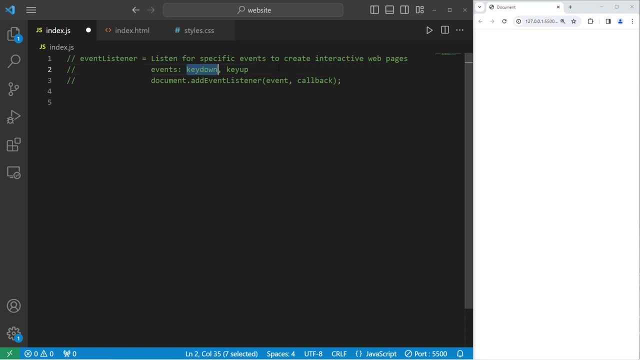 so you should avoid using key press. A key down event occurs when you press down on a key. A key up event occurs when you release a key. By adding an event listener to the DOM document, we can detect when we press down or release a key. Here's how We will access our DOM. 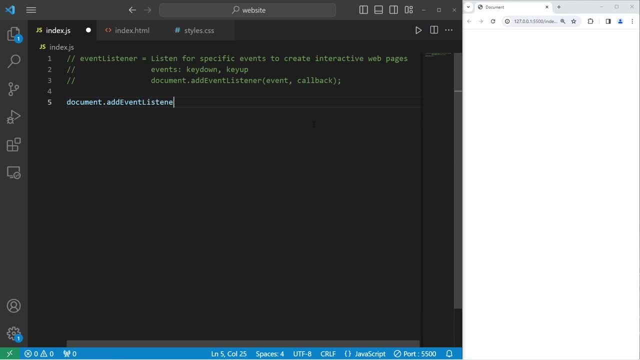 then add an event listener. Add event listener. We have two arguments: The event type and a callback. When we press down on a key, let's do something, Doesn't matter what key it is, Any key. For this next argument, I can either pass in a callback. 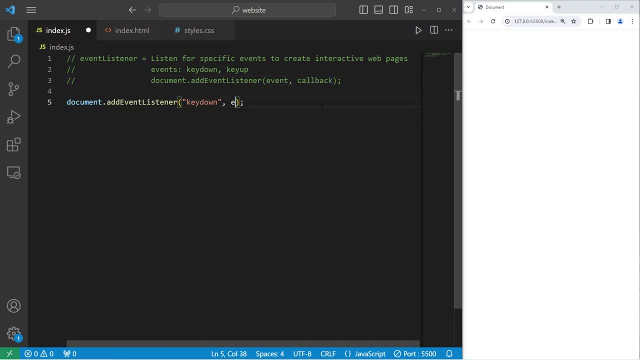 an anonymous function or an arrow function. I like arrow functions, so I'm going to use an arrow function. We're provided with an event parameter. When something happens within our web browser, an event object is created, We can access it. So I'm going to consolelog. 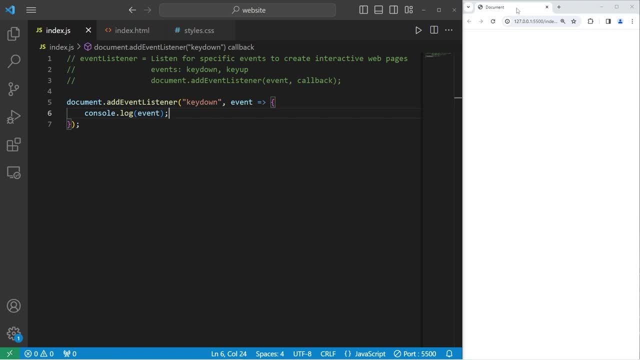 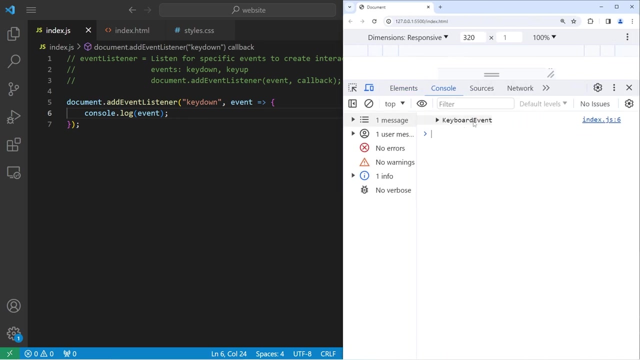 this event object and we'll see the details. Be sure to select your web browser. I'm going to press the Q key, Then let's go to inspect console and here's that event. The web browser provided us with a keyboard event. 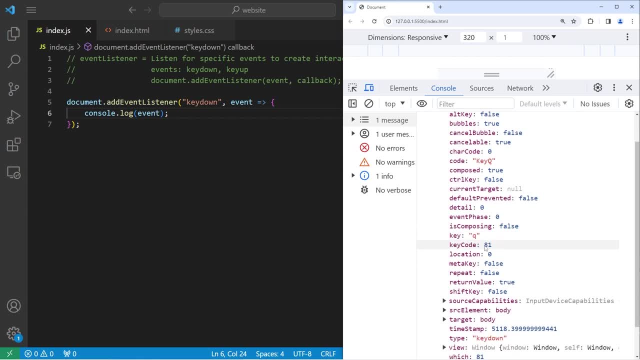 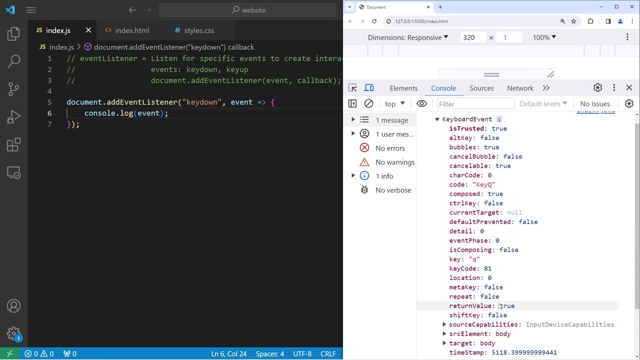 The key pressed was Q. There's a relevant key code of 81. And there's other properties too. like was the alt key being held down at the time. It wasn't Same thing with the shift key And the target, Which is the body of our document. 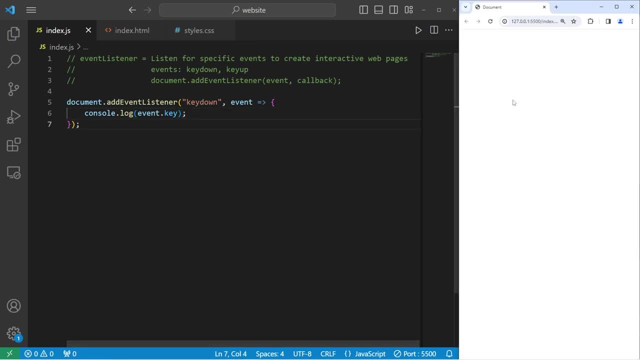 I'm going to output the key property of the event. We'll press a different key. I'm going to hold down the F key. I'm not releasing it, I'm holding it down. We're going to consistently fire key down events. 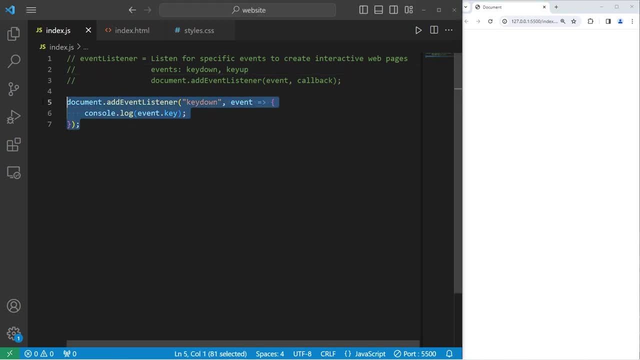 I would like to detect when I release a key. I will use the key up event. So let's copy this, paste it. The event is going to be key up. I'll display something else. I'm going to use a template string. 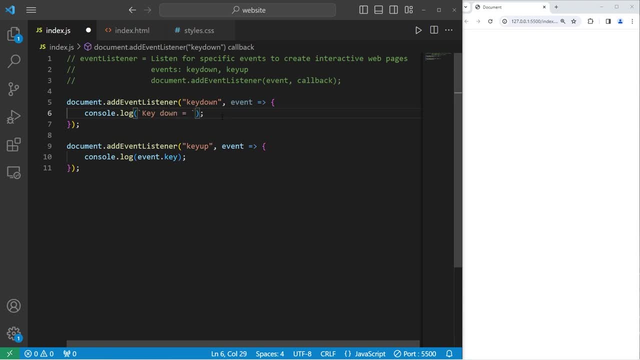 I will display key down equals. Then I will display this event's key. Let's do this with key up too. I'll just copy this Key up: equals- event dot key. Let's go back to our console. I'm going to hold down the S key. 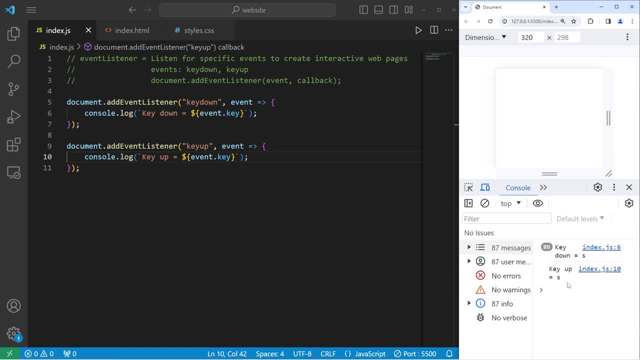 Then, when I release it, we'll have a key up event. Key up equals S. Oh, one more important thing: The arrow keys. We have arrow up, arrow down, arrow left and arrow right. If you ever would like to make some sort of game, the arrow keys are also accessible. 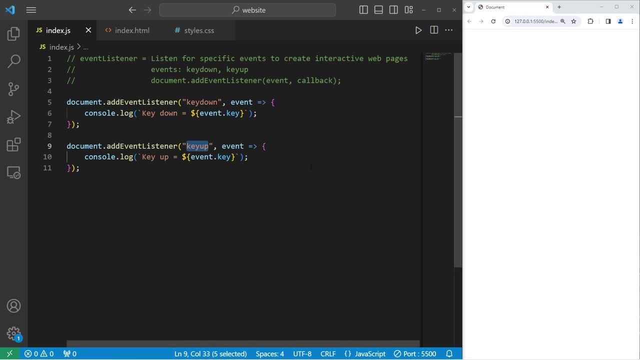 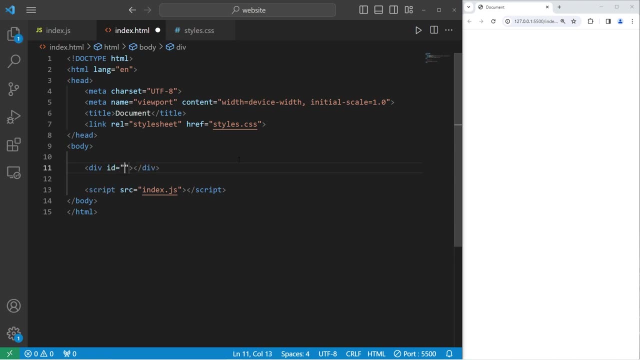 Now what we'll do on key down and key up is change an HTML element. So to make this simple, within our HTML document I'm going to create a div element. This development will have an ID of my box. I'll add some text, An emoji. 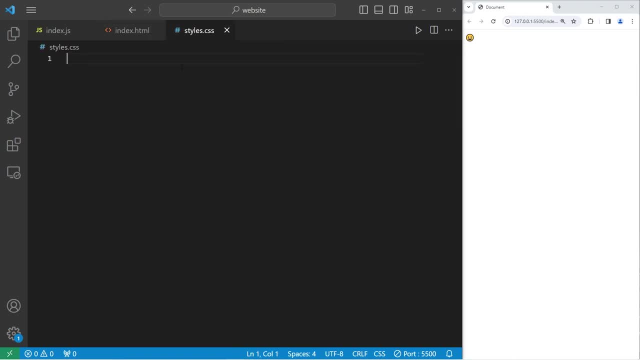 Alright, let's add a little bit of CSS. We will select my box. I will set the background color to be light blue. We haven't picked light blue yet. I will set a width of 200 pixels, A height of 200 pixels. 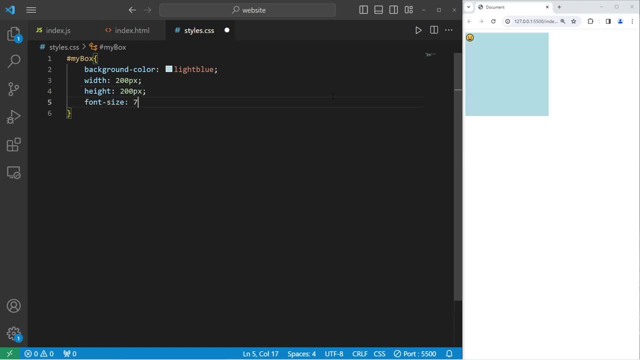 A font size of 7.. A font size of 7.5.. REM, I'll use flexbox, Display, flex, Justify content center. Align item center. This part is important for the next exercise. We are going to set the position to relative. 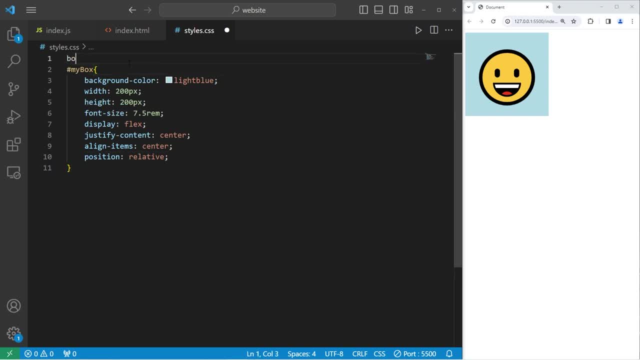 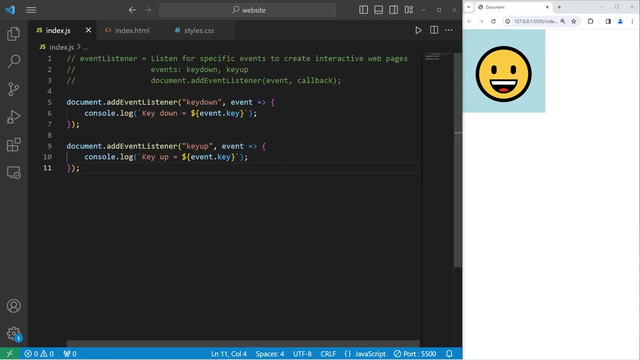 For relative positioning. I'll set the body of my document to have no margin, Margin 0.. Alright, we are ready. We are going to select the ID of my box. const mybox equals documentgetElementById. The ID that I'm going to select is my box. 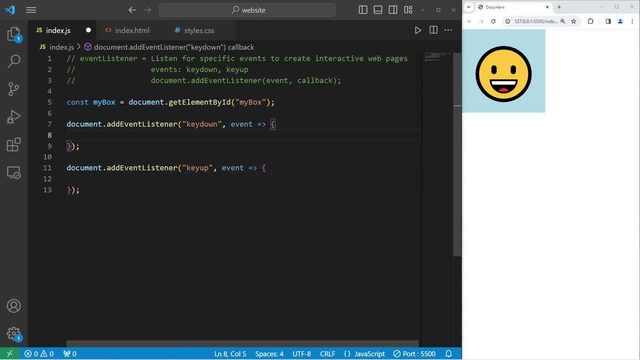 When I press a key down, I'm going to change the text content of my box: myboxtextContentgetElementById. myboxtextContentgetElementById. myboxtextContentgetElementById. myboxtextContentgetElementById. myboxtextContentgetElementById. I'll pick a different emoji. 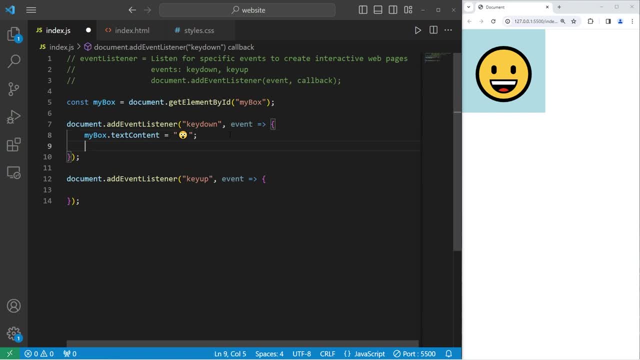 Let's do that one. I'll change the CSS. myboxstyle backgroundColor equals Tol. When a key is pressed, the CSS has been changed. I'll release that key. Let's not revert to normal HTML element. stays that way. 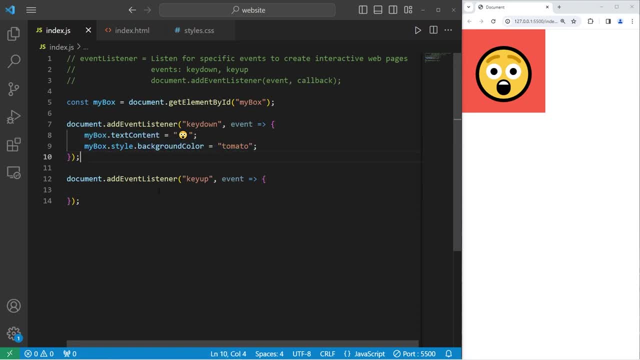 What we'll do is that when we release a key, we'll revert these changes by going back to the original. So let's take my box, change the text content to equal and emoji. because I like emojis, We'll use the original one. 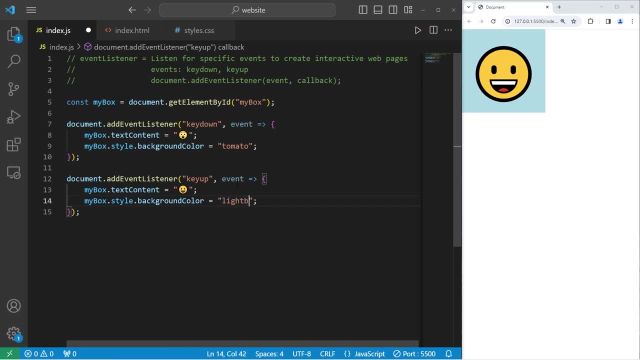 Then I will set the background color to be light blue. Now, if I were to hold down a button, the HTML and CSS is going to change until I release that button, which I am about to now in 3,, 2,, 1, go. 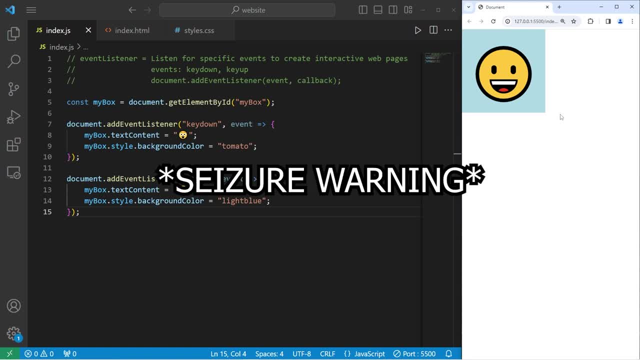 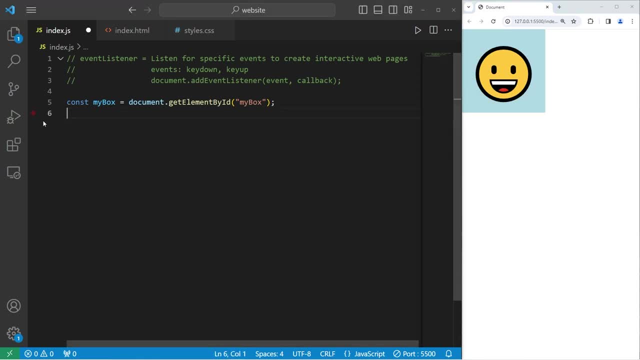 I'm going to try and press the spacebar as fast as I can. Seizure warning. Let's gooooooooo Okay, it's about time we move on. What we're going to do now is, using the arrow keys, move this element. 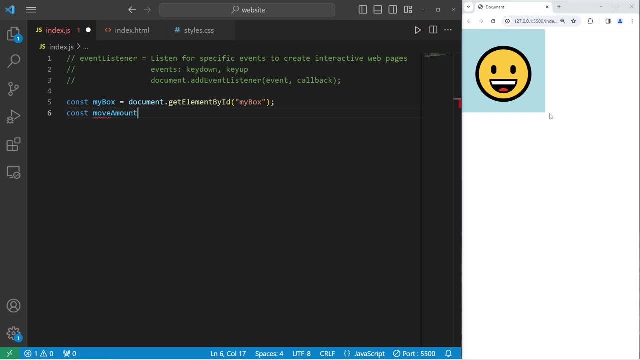 We're going to create a const of move amount When pressing an arrow key. how far do we want to move this element? Let's say 10,. for 10 pixels, I will create a variable for x. think of these as coordinates. 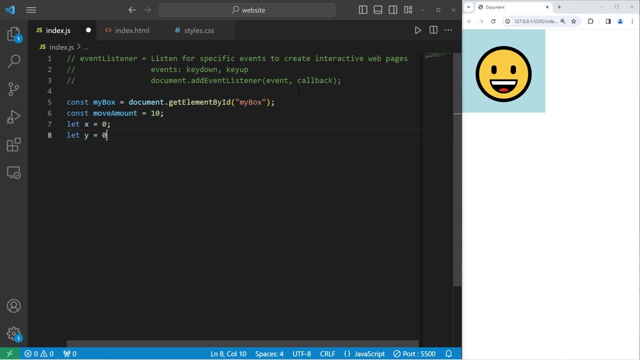 I will set that to be 0, and y. y will also be 0.- X for any horizontal movement and y for any vertical movement. Document dot. add event listener When we have a key down event. I would like to do something. 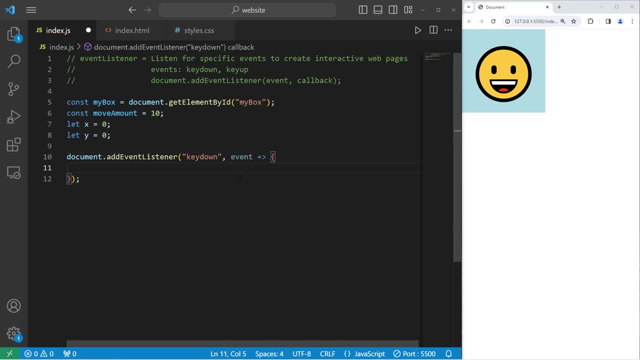 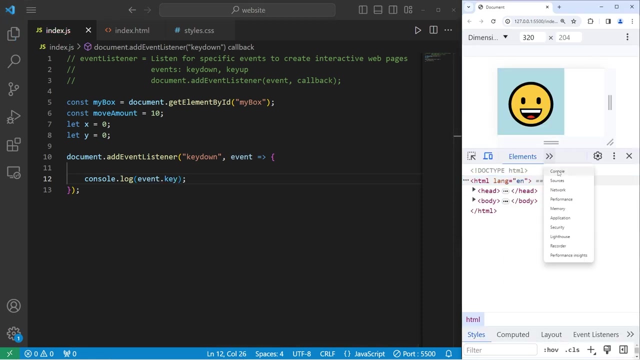 I'll write an arrow function. we're provided with an event. do all this code. I only want to do something if a user uses an arrow key. So if I was to console dot, log my event, then access the key property. Let's go to inspect console, select your document. 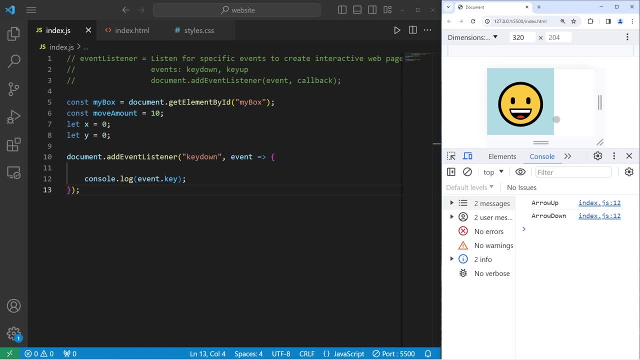 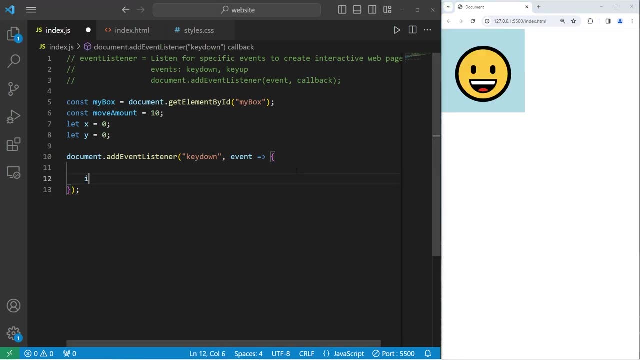 I would like to do something only if the key pressed is arrow up, arrow down, arrow left or arrow right. I don't want any of the other keys. I can write the if statement. If Access our event. Okay, If the event access its key, follow this with the starts, with method: does this key? 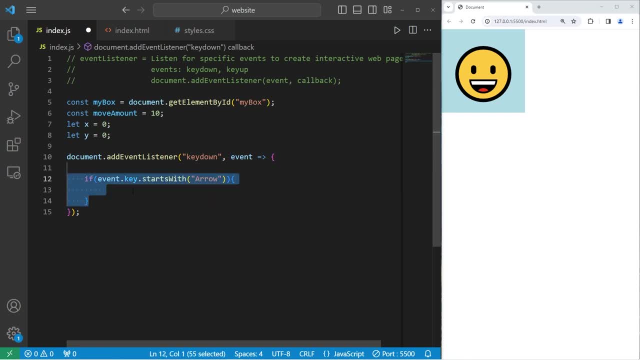 start with arrow. We'll only enter this if statement, if the key of the event is arrow up, arrow down, arrow left or arrow right, Then we'll write a switch. We haven't written any switches for a while. We will examine the key of our event. 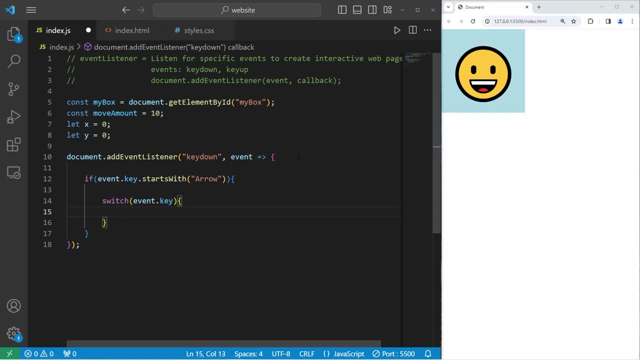 With switches, we examine a value against matching cases. If we have a case of arrow up, if the key of our event matches the case of arrow up, then do this. We'll take our y coordinate, subtract our movement amount, which is 10.. 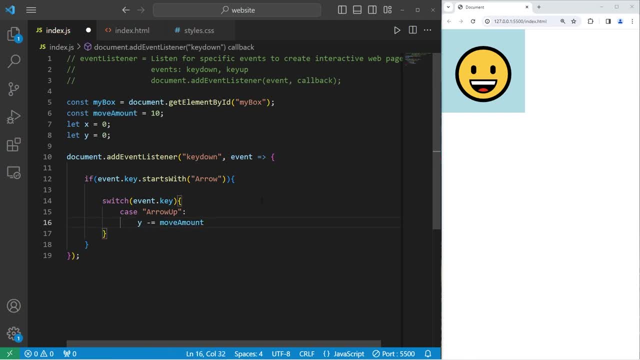 Y minus equals the movement amount, And then be sure to break, to break out of the switch. Then we need a case for arrow down, Arrow down, Arrow down. Y plus equals our movement amount. Arrow left, Arrow left: X for the horizontal axis. 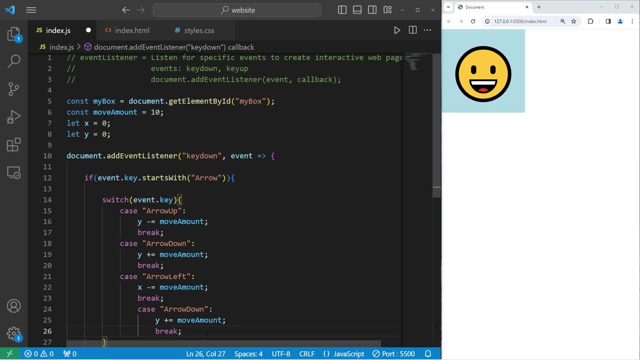 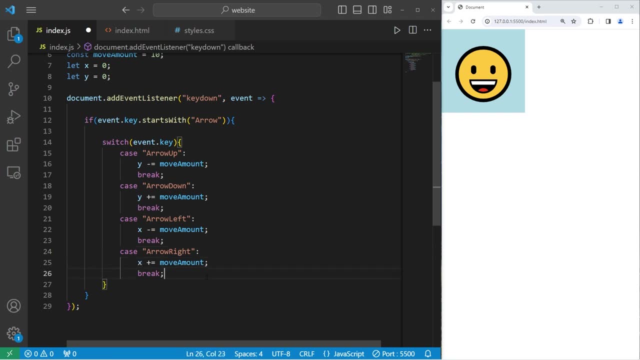 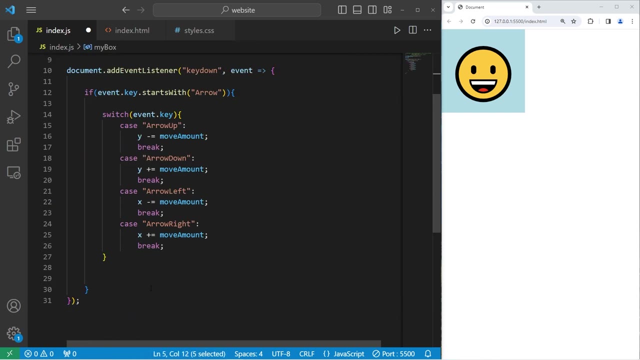 Minus equals the movement amount, And then arrow right, Arrow right, X plus equals the movement amount Then outside of the switch. So our slope and its look are the same as two elements with the same count as once. We're golden. 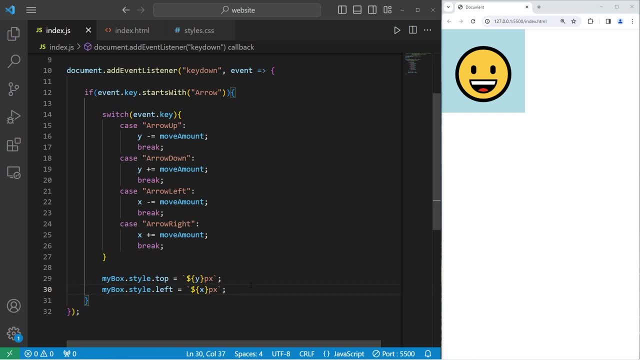 We're out of our element spaces. So what we need here is we need to time Jesus, Create a box. We must have the Y coordinate. The Y coordinate is one x in pixels. Be sure to select the body of your document. We can move right with the right arrow. 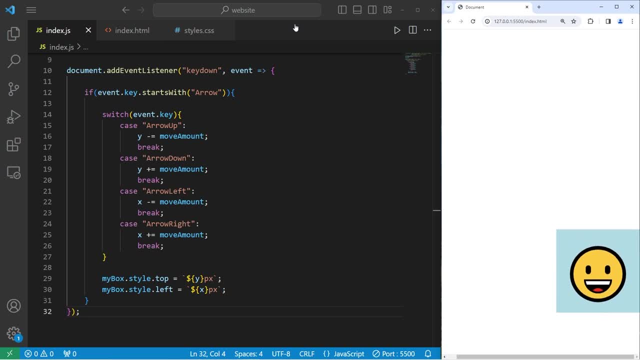 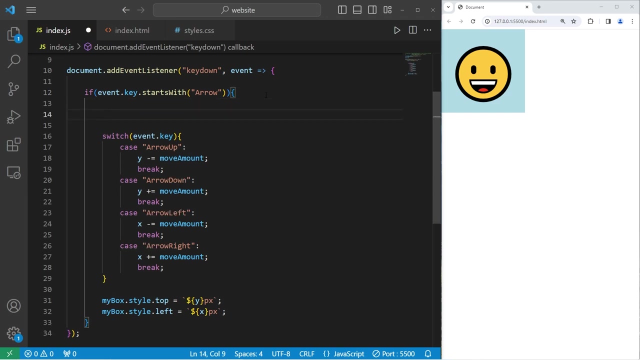 key Down, left and up Or diagonal. if I hit two keys at once, The arrow keys have a default behavior to scroll. You can see that if we go down too far we have a scroll bar on the right hand side. We can prevent the default behavior of a key. We just have to add this line of code: Take: